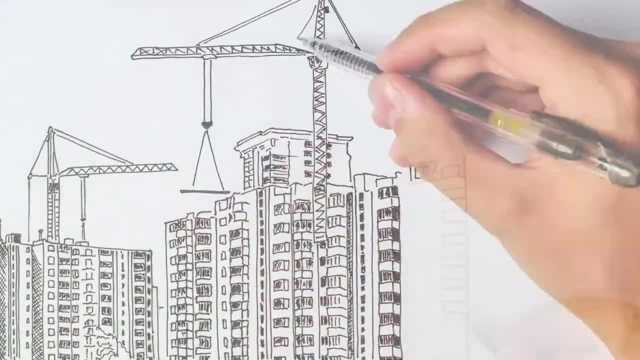 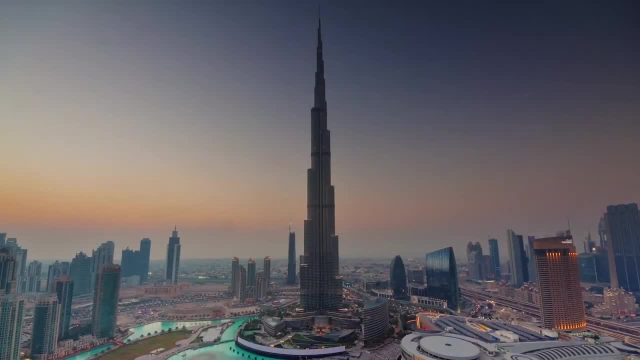 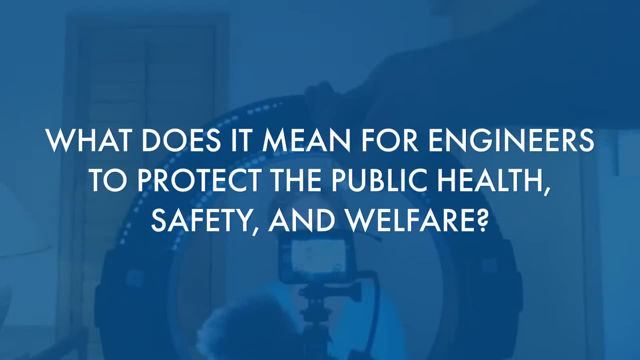 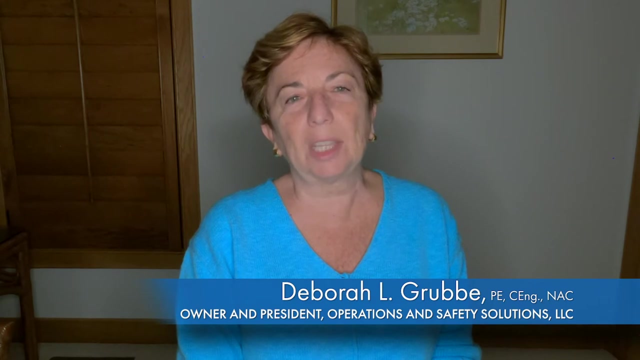 than any other professional, and the reason for this is we create things that are going to last 50, 100, you know- sometimes even a thousand years, and they've got to be safe throughout the entire duration of their life. the public has a right to be able to get their products made in a safe manner. the public has. 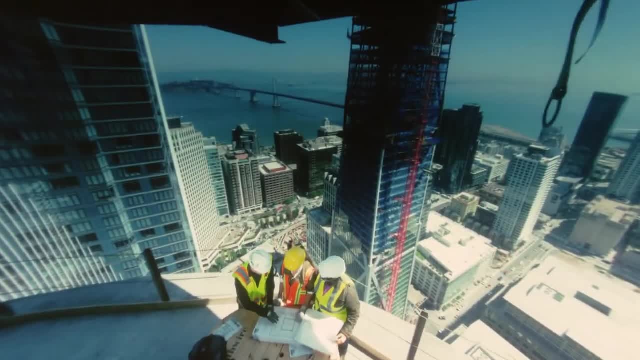 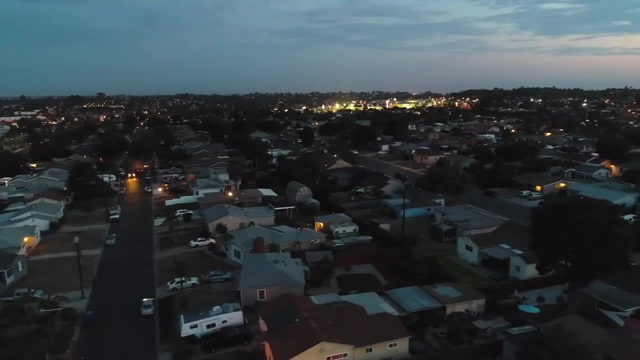 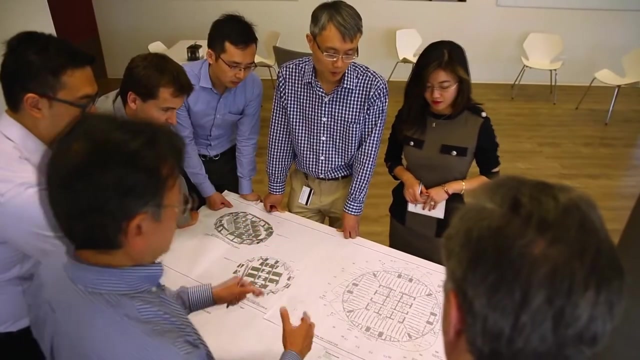 a right, and the workers have a right to not expect any serious issues. when you go to sleep every night in your home, you just assume that the building is going to last through the night. there's not even a question about it. and if I look at what is important when it comes to ethics, it's very clearly. do you understand? 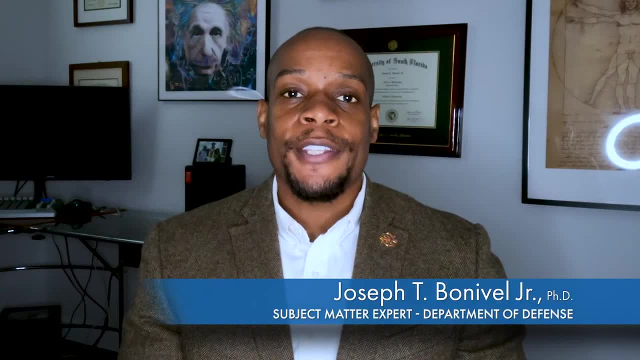 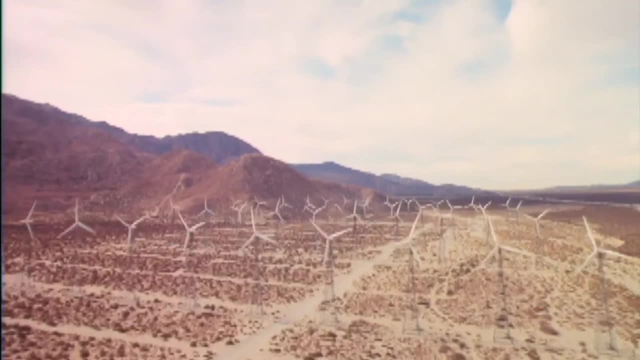 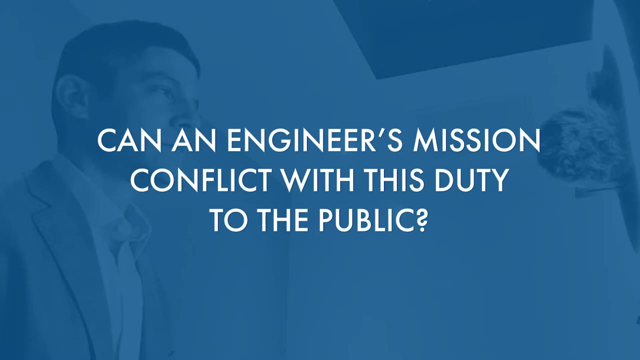 right from wrong. engineers in general want to advance human society and because we want to do that, we want to help mankind. ethics plays a very important portion in ensuring that you're helping and not hurting those around you. the problem is that next to mining, The problem is that next to mining. 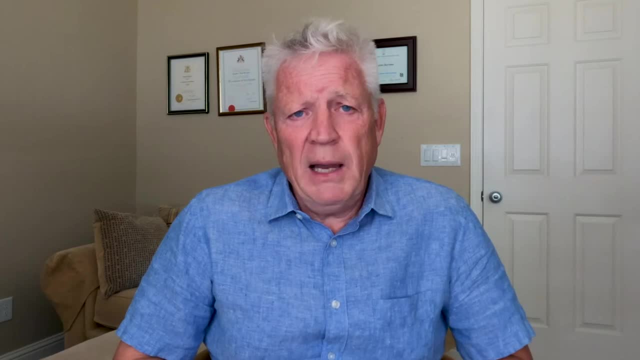 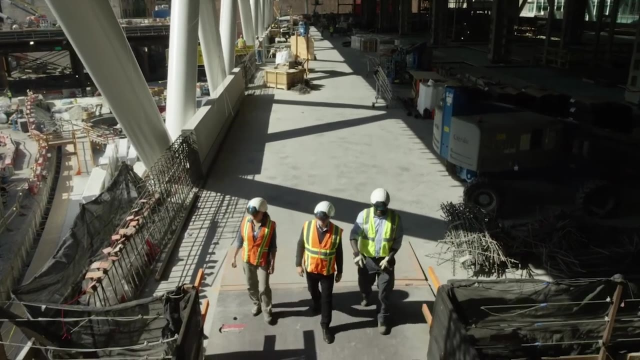 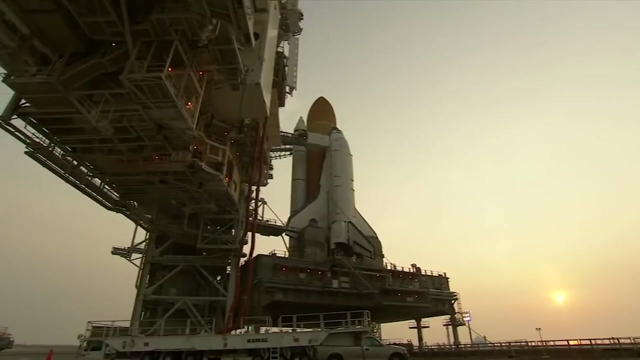 there are more deaths in construction than any other industry on the planet. there's an opportunity. when large sums of money are involved, there is always an opportunity to do the wrong thing and it is never right to do the wrong thing. if you have good ethics, you, you will have a good safety culture. 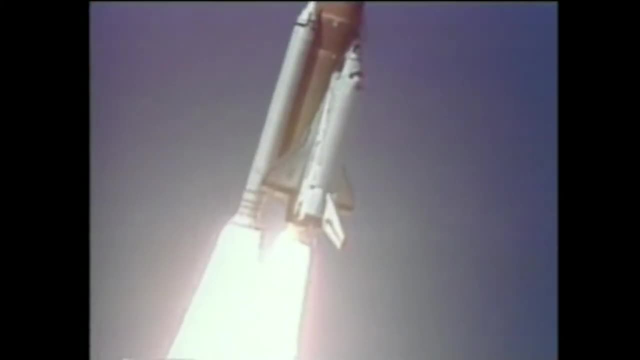 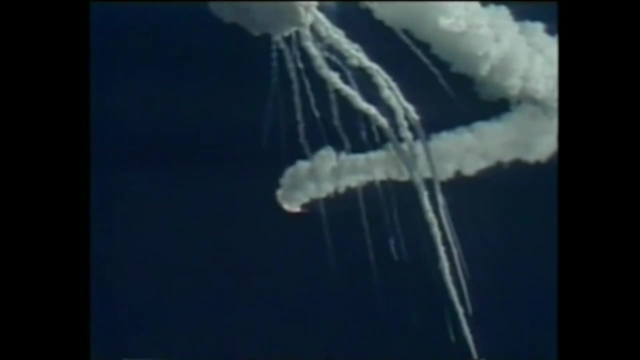 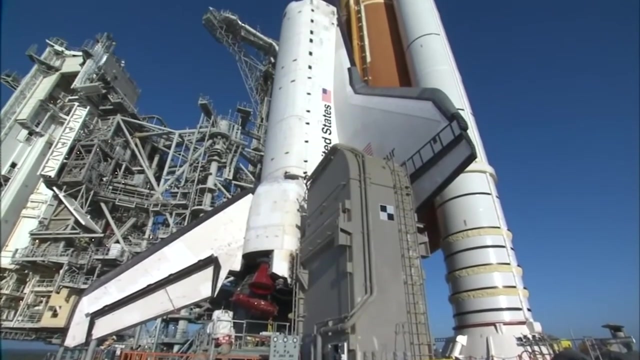 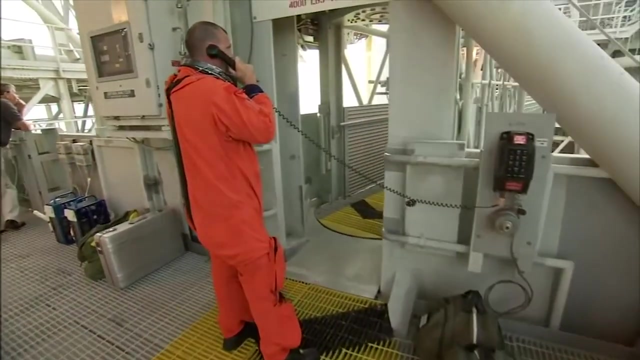 what happened in both the challenger and the columbia were similar failure modes. it was just a different item of the shuttle. people knew that there were issues, but they were unable to raise their concerns. if anybody has any concern about anything at any point in time, please bring it forward. 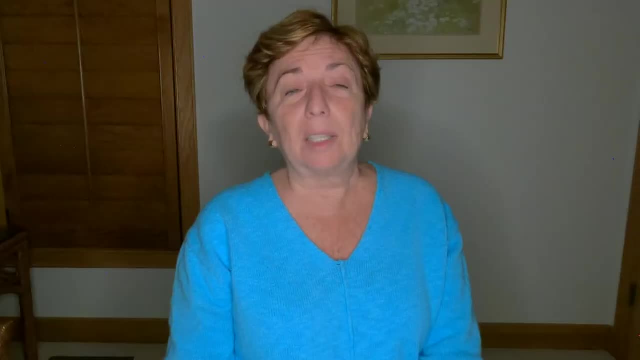 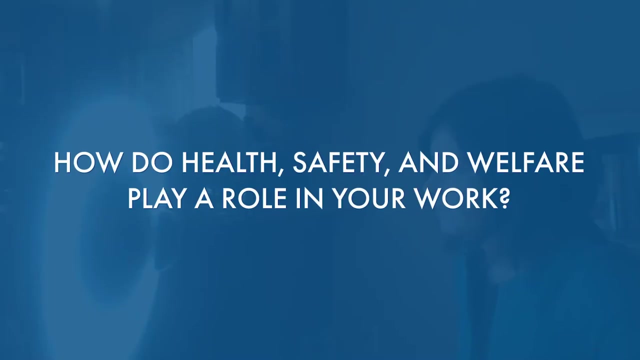 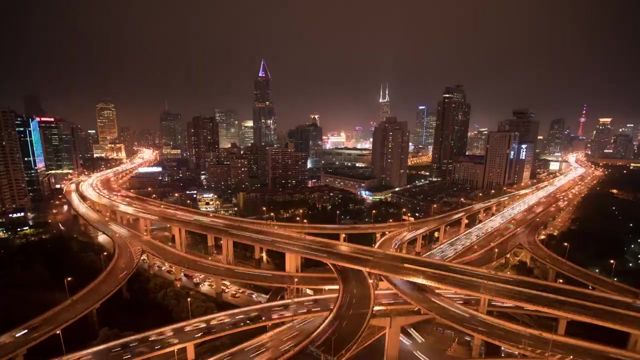 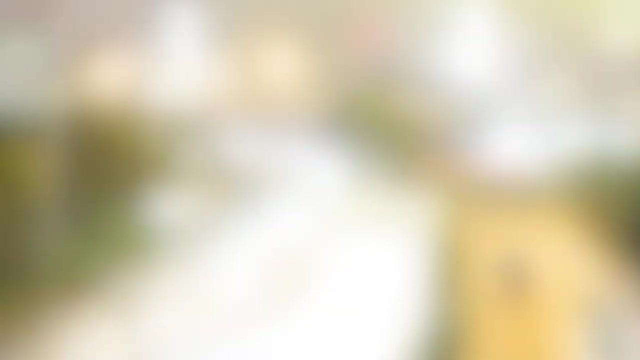 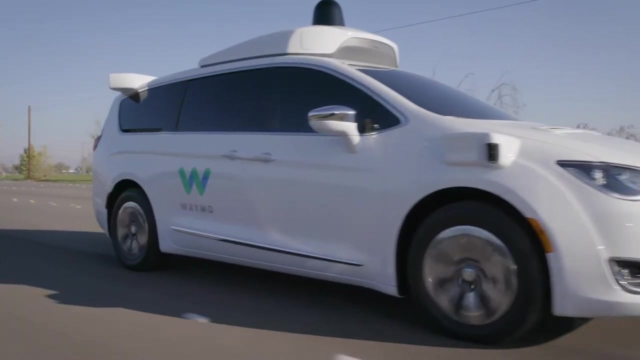 because good news is bad news, delivered early enough to do something about it. people have been driving cars for the last hundred years. however, what we know is that we lose over one million lives every year worldwide to traffic fatalities. autonomous vehicles have the potential to save millions of lives. self-driving cars- uh, don't get distracted. they don't get drunk. they. 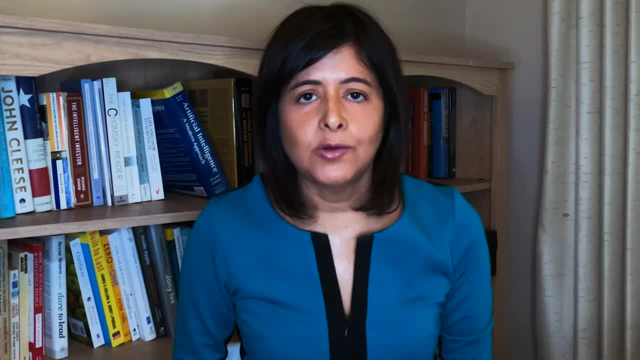 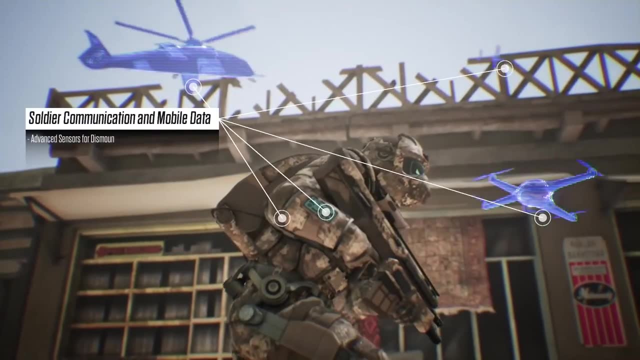 don't get angry. an ethical approach is central to what we do at wemo and it's a huge power point for us what we do at Waymo. One of the more interesting projects that we have is the exoskeleton project. It's very similar to what folks have seen on video games, where we want to make our soldiers stronger. 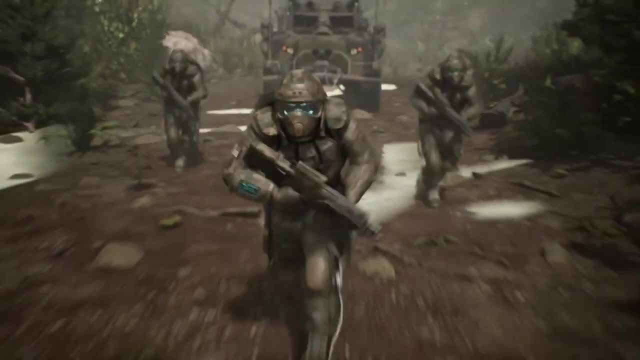 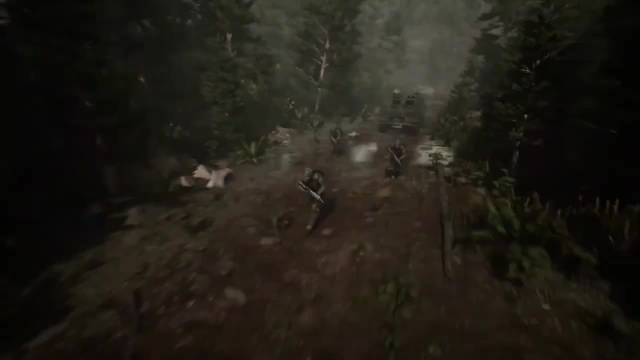 faster and able to see the battlefield in a more efficient way using virtual reality. That is one of the coolest projects out. It's one of the things that's going to be cutting edge and it's one of the things that's going to save soldiers lives At. Dimension Inc is where I work as an 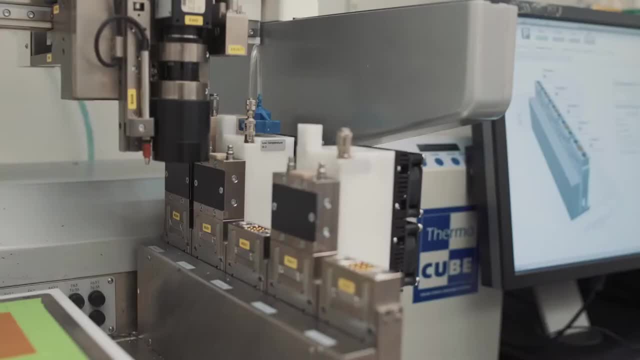 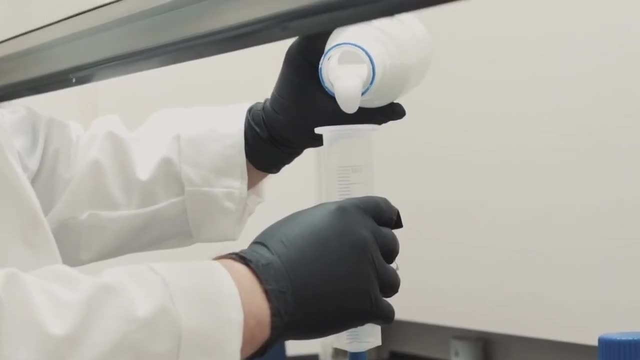 engineer. We are developing materials and 3D printing structures out of those materials that go inside the human body. That's a very big level of safety. We go through extensive biological testing and we need to pass those tests. We need to show that, whatever we're, 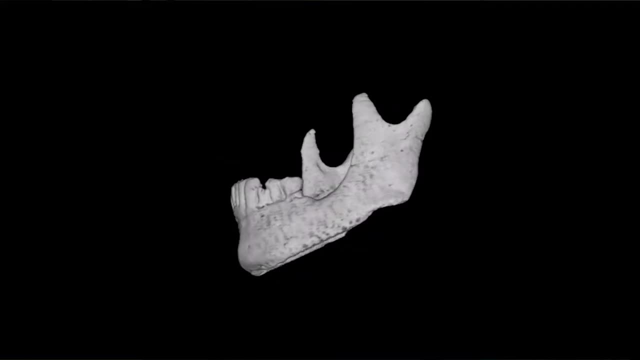 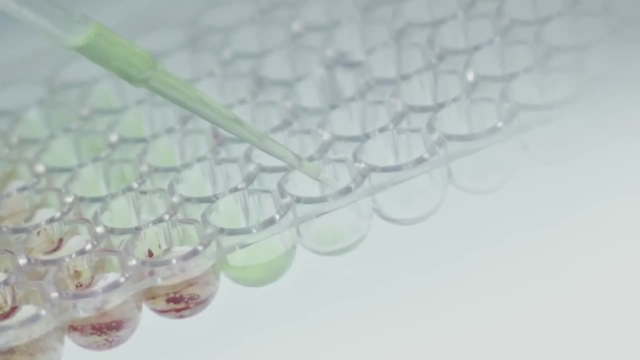 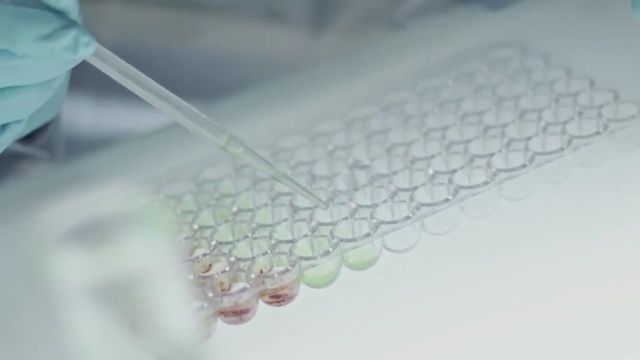 making is safe long-term inside the body and that it can also be properly used by the doctors and the surgeons who will be the ones putting these things inside people. If I think about COVID, I know chemical engineers right now that are working to bring a vaccine to all of us. 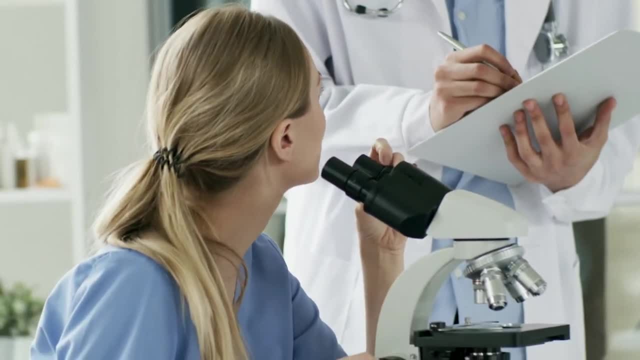 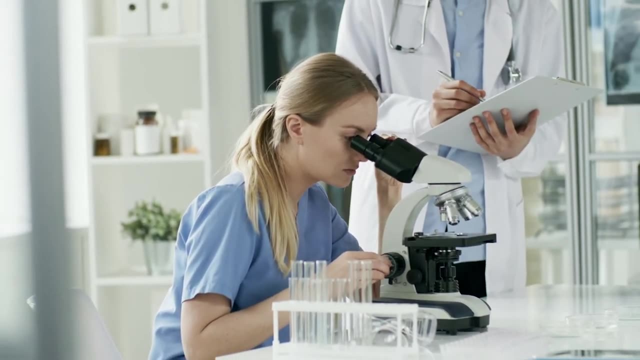 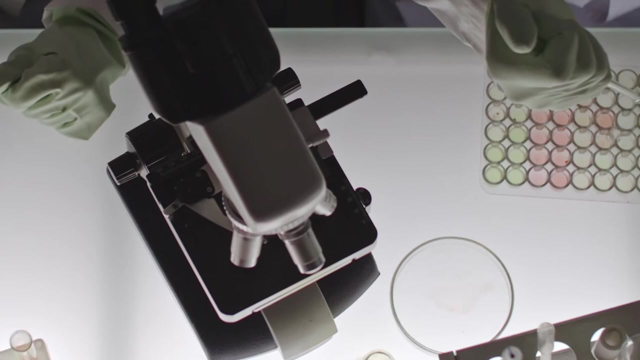 Chemical engineers are involved in every phase of the vaccine, from the creation, the idea of where does the substrate of the vaccine come from. The chemical engineer will also be engaged in separating any impurities that may show up in the vaccine, so that you get the most efficacious drug that you possibly can. 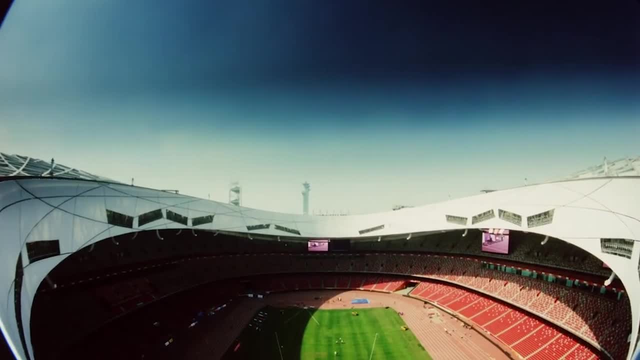 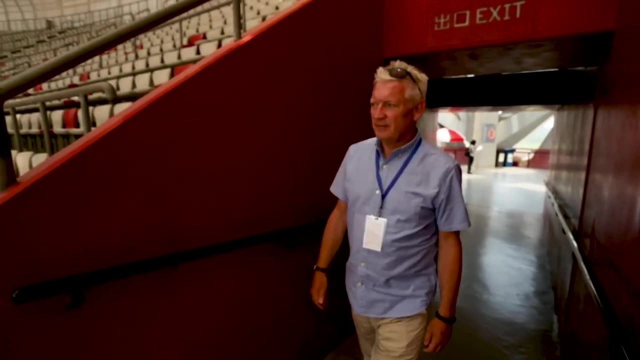 The Bird's Nest Stadium is one of my projects. So one of the big challenges of a project like the Bird's Nest Stadium is: you're going to have an event. the whole world is going to see it. There's going to be 100,000 people or more inside the stadium. It's got to be safe. 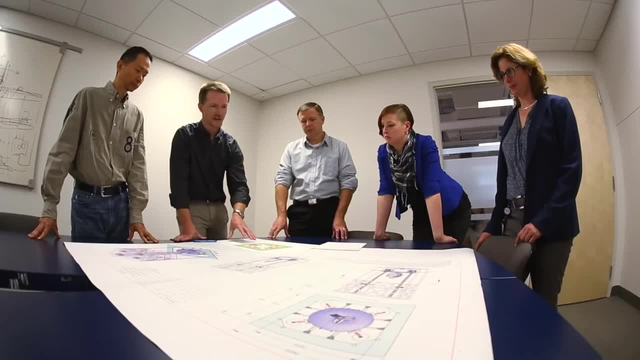 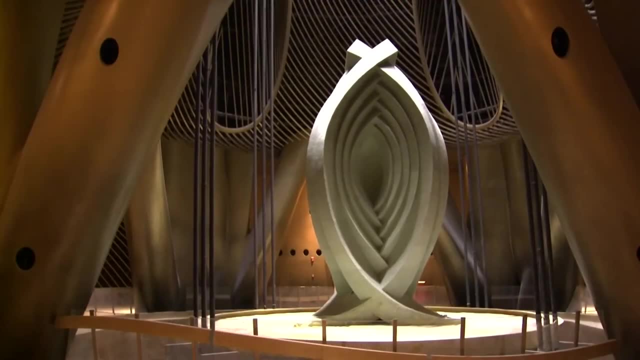 An engineer is the linchpin and we make sure that at every step we have a factor of safety in there. We want to understand what that factor of safety is. We want to understand if it's, If this goes wrong, how can we ensure that no one is going to get hurt? 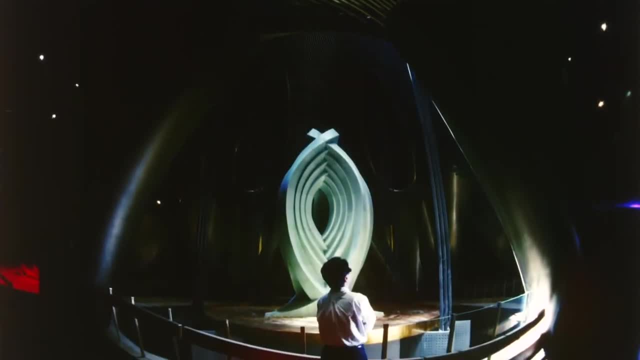 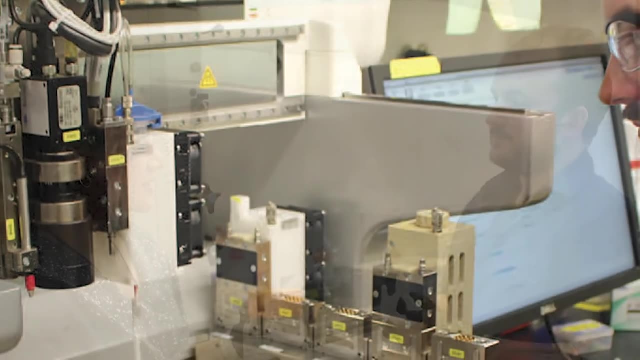 Without an engineer in the room, you are planning to fail. You know I was driven by not only my curiosity for science and engineering, but wanting to apply it to make people's lives better. At the time when I got into the field I didn't know to call that ethics. 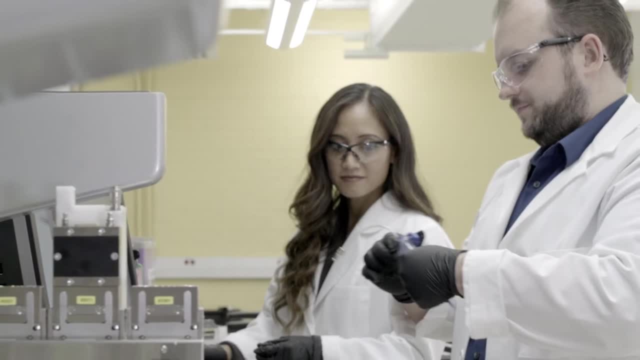 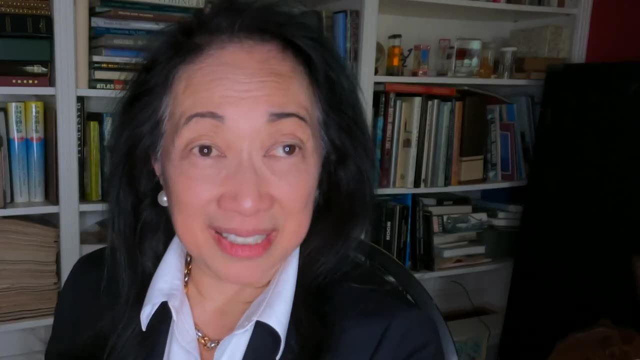 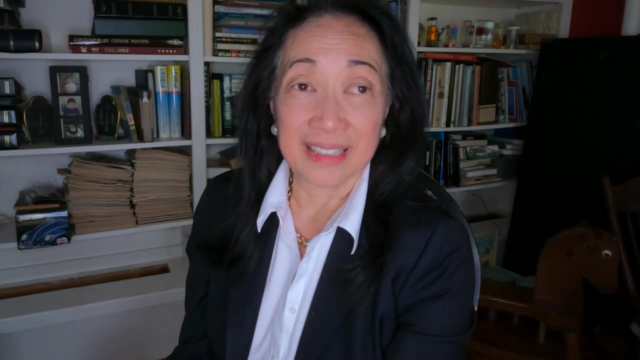